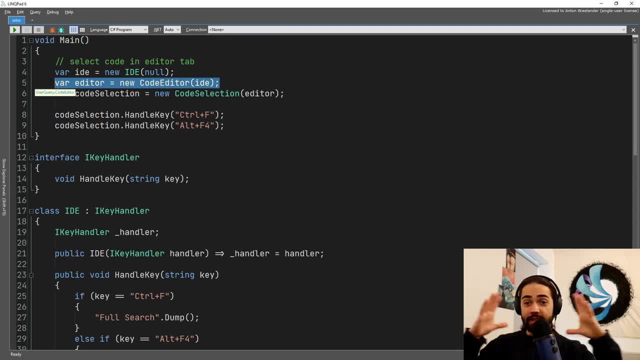 and you now have code in it. So this is the code editor, this is the editor window. You can have other windows, like the terminal task management solution window output, all sorts of windows, right, You can have the settings, windows, etc. 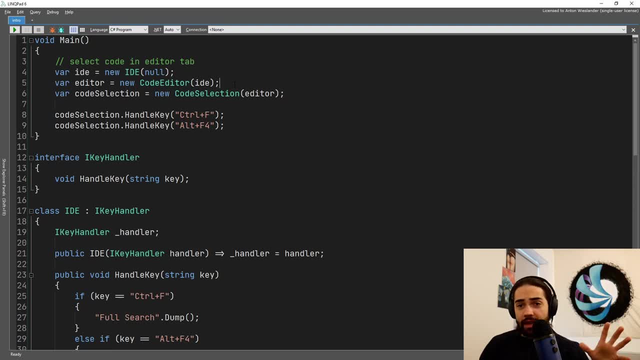 Let's focus on the code window. So once we have the code editor open, what we can do is we can then select text. okay, And this is what I'm going to refer to as the maybe context or focus context. basically, What context are you currently in? Are you in the context of just the IDE? Are you in the 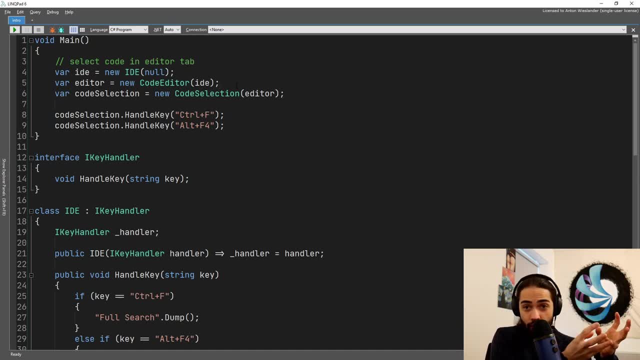 context of the code editor, Or are you in the context of selecting some piece of code or highlighting it, or just having your cursor on it? The chain of responsibility is the layers or the context within the IDEs. The event that we're going to be handling is the key. 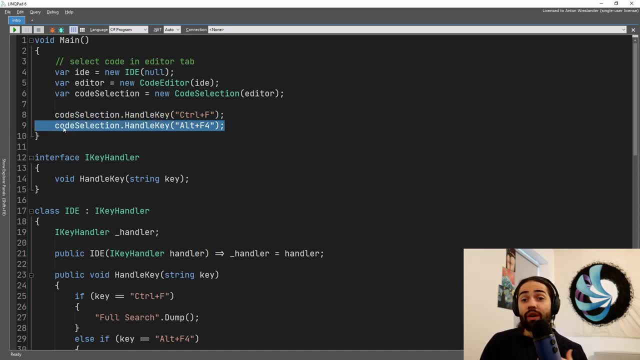 input. We all know the LTF4 key input. Wherever you are in your program, you press LTF4, it's going to attempt to close your application, right? If you play video games, multiple people will troll you. they'll press LTF4 for whatever and when you're young and you press it and you're like 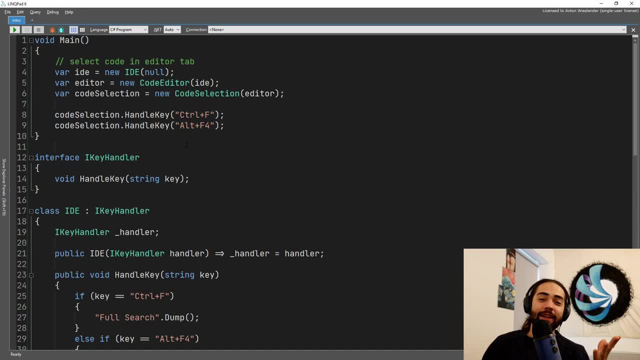 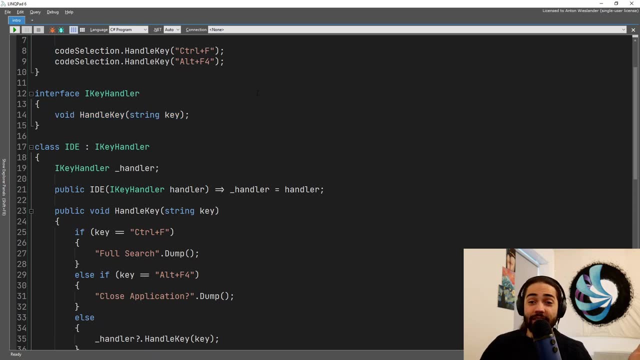 oh man, close my video game. Anyway, a little bit for the structure of how I've set this up. we have the IKeyHandler interface, really simple. We're just going to handle a generic key. You can have your generic request, event message, whatever accepted in the whatever is going to try to handle. 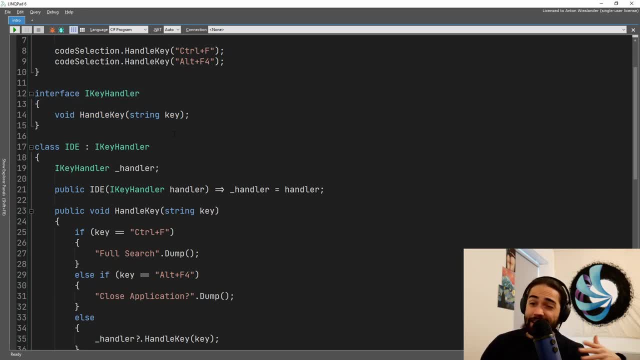 this message. This may look a little bit like mediator, and the mediator library can be used to implement a chain of responsibility as well, And we'll take a look at an example later of how this works in ASPNET Core. So we have our first IDE implementation. 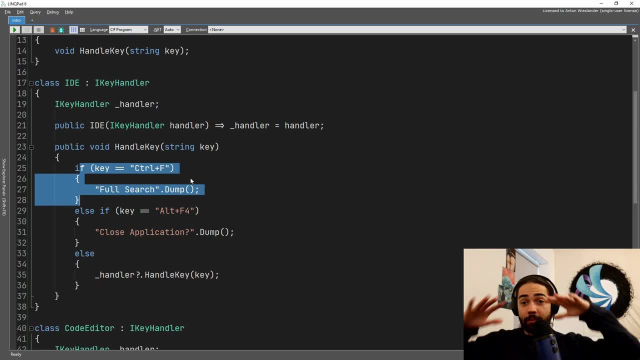 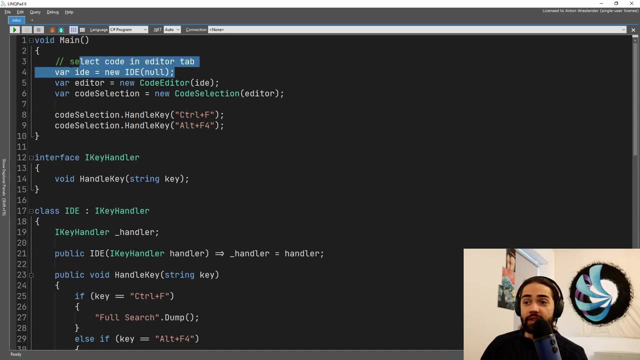 Where, if I press Ctrl F, what's going to happen is I'm going to do a full search on the ID, So that means I'm going to search files. I'm going to search text within files. it might try to find some options. Or if I press LTF4, it's just going to close the application. Okay, so this is when I 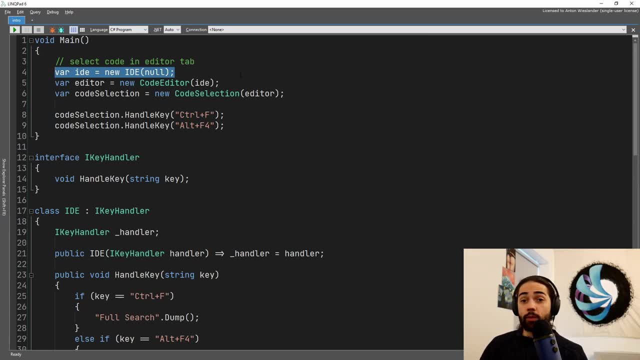 create IDE. Then if I focus in on the code editor window in the background in the code, I can say we have our initial root context of IDE when we've loaded up the application. Now that we're clicking on the code editor, let's create this new code editor object and let's put the 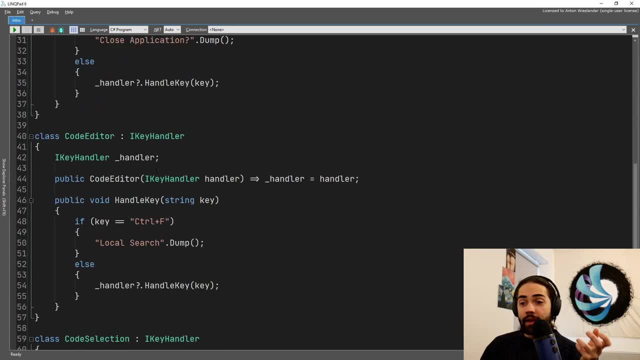 IDE in there. So now we're in the editor context, And in the editor context again, it's a key handler. You're going to press keys in there where you're either going to type the code that you are typing or, if it's a 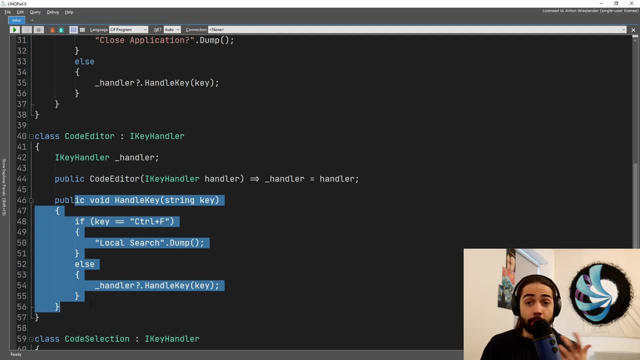 special key bind. we want to handle it. LTF4 is not part of this, although we could still handle it technically in the code editor. We just choose not to. But anyway, you can press Ctrl F inside the code editor And what's going to happen? 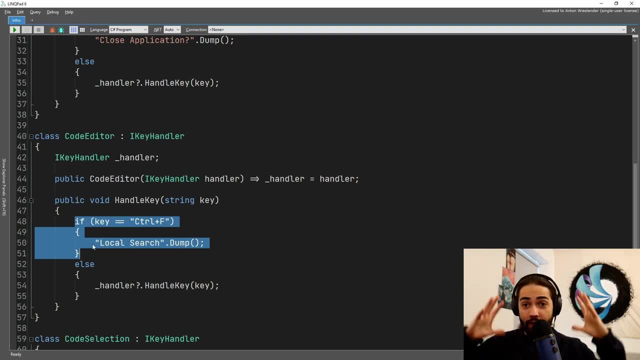 happen is you're going to search only the code within the code editor. You do not get access to the outside scope of the application, right? So you do not search the files. you do not search the code in other files, you only search the. 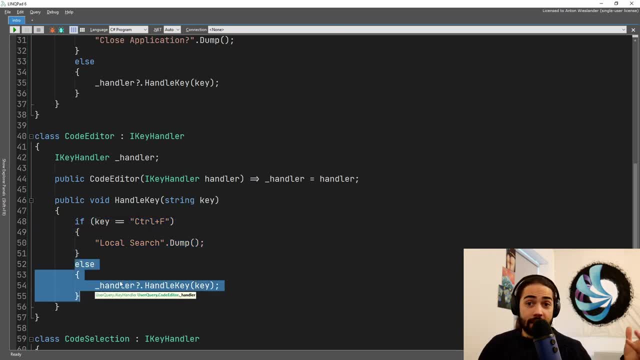 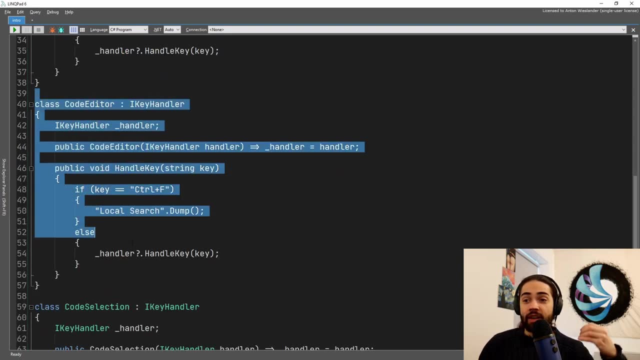 file that you're currently in, And otherwise, if it's a keybind like Alt F4, it just goes and gets popped back into this ID, right? So the chain of responsibility here is code editor first if code editor doesn't handle it. 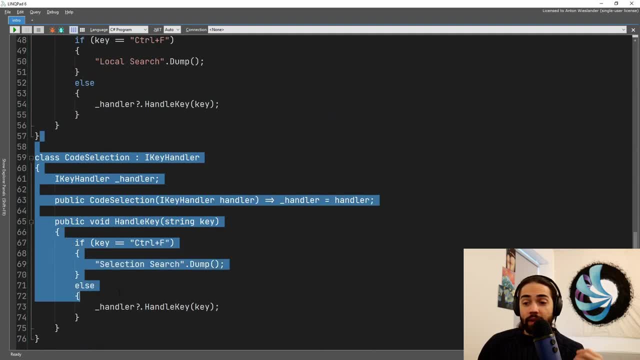 it goes back to the root, to the ID, and then we can have the code selection. So we select a piece of code. I don't know if you've ever done it. you may have multiple methods within your file. you want to replace specific things within. 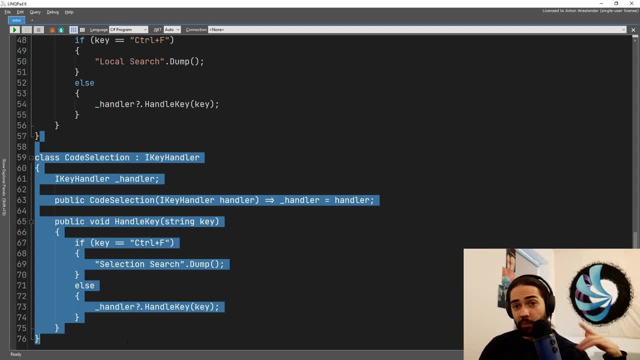 one method. you highlight the method. you press ctrl H- that would be in Visual Studio to find and replace- and then you type in the search term that you want to replace and then what you want to replace it with, and it will only. 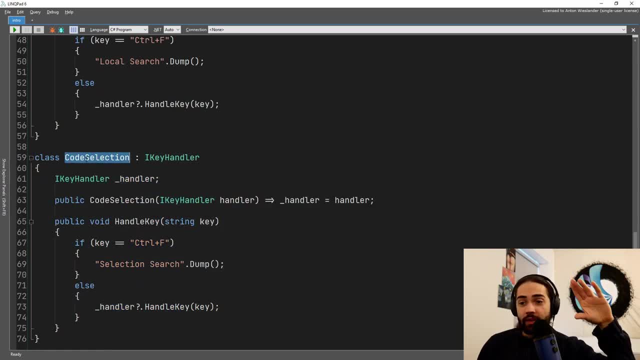 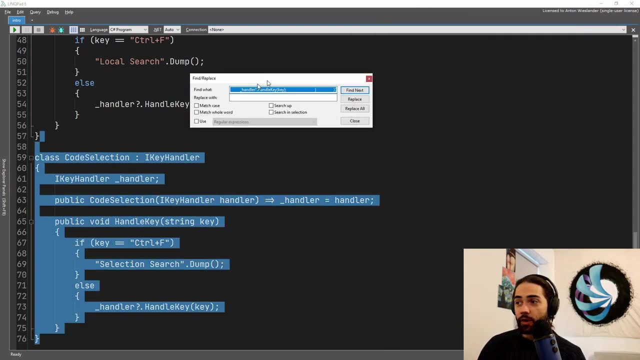 affect the selection. So this is the same thing. So code selection. once we've dragged our cursor over the code like so and we press ctrl F, you can see there is an option here: search and selection. Let's hypothetically think that if I have code selected it's gonna bump up the context. 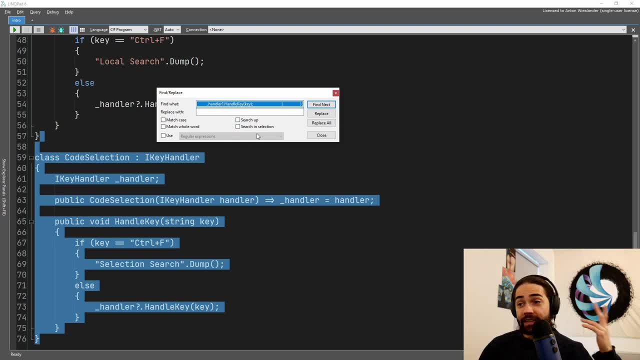 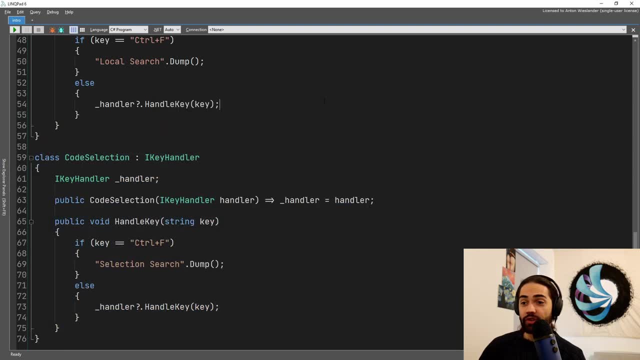 I press ctrl F and it should automatically tick this search and selection option for me. Okay, instead of just popping up the window as if I was just doing a regular search, You can see also from the original code selection. it is actually filling out what I want to search for. If I don't, 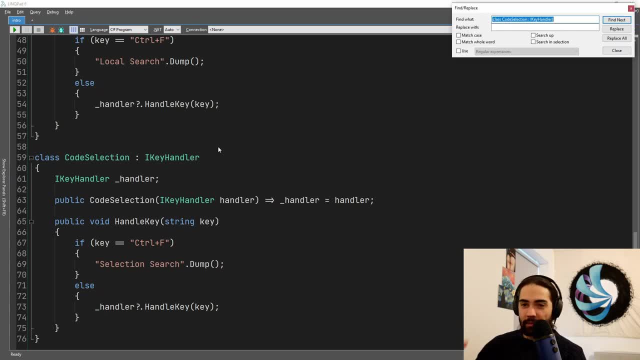 have anything selected. it should be empty, right, but it's just bringing in the previous one. Hopefully you get the picture. Something happens, a request, message, event, and then you have to handle it in some way, Being able to. 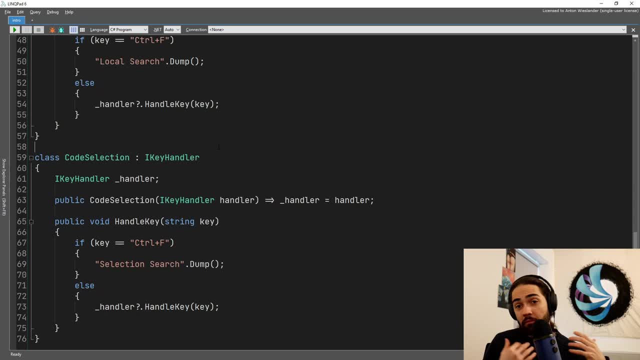 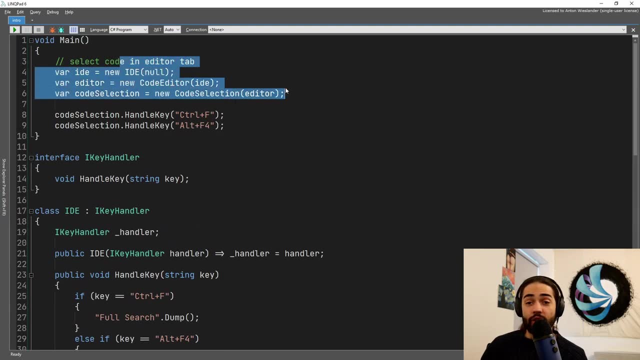 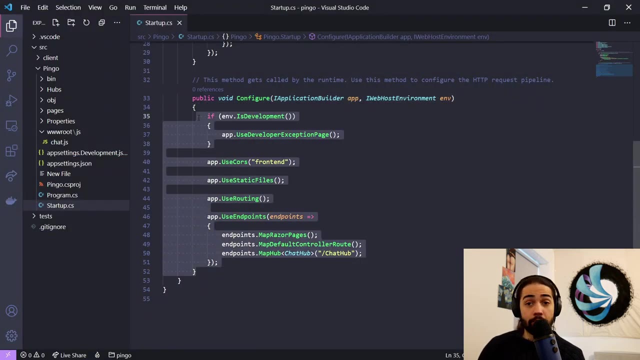 dynamically compose how you're going to handle requests or messages is the whole you know shebang chain of responsibility. Here we can dynamically compose context within our application. in ASPNET core environment This may look more like a middleware pipeline. We have a HTTP request that comes in at a certain 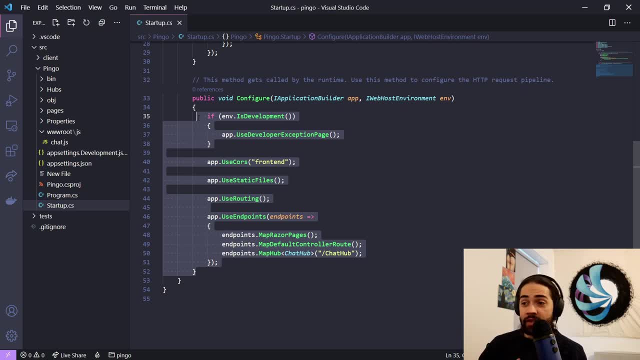 address the path, the query, the headers. They're all gonna affect what is going to happen, So it may look like it's going to different routes. it's, you know, going to path slash API, slash cars or slash API- slash animals. That is a. 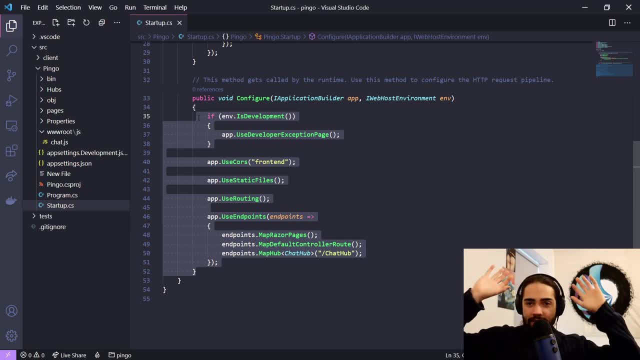 little bit of an illusion. that is a random 한국 말, how the middleware basically takes the path and it then routes it to the correct action. what really happens is it all hits the same socket, the same endpoint, all requests go to the same host, to the. 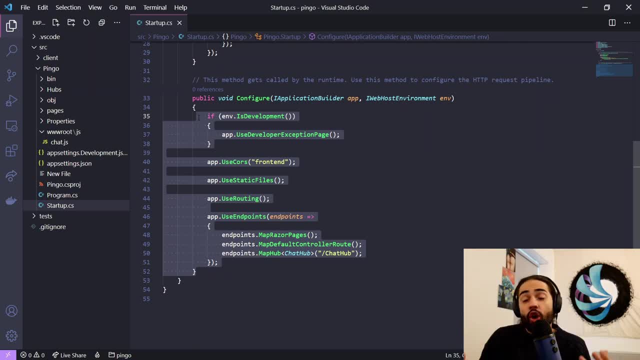 same port. your application then says: all right, what context do we have? and in this case, the context is going to be: what path? so if the path is prefixed with static or is a stat, it points to a static file that we can actually find in our www root folder. just serve that right. all good chain. 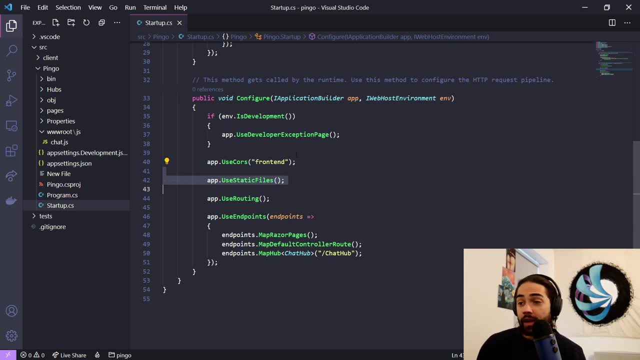 of responsibility. first thing, to handle static files. cool, if we don't have course enabled, we might just say: oh, this is coming from some different domain, get that, get the hell out of here, right? uh, we, then we can then say things like: all right, is this meant to be a razor page? that 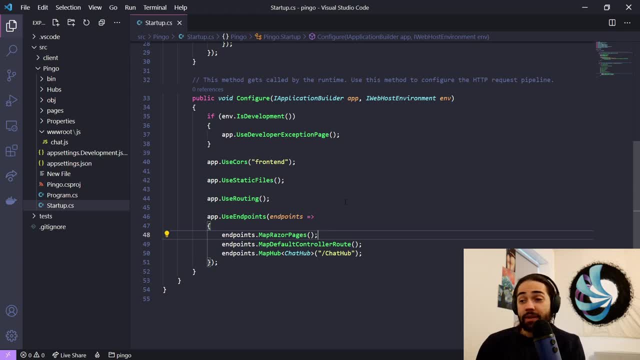 we registered, is this a controller? and for the dynamic side of it, let's say you're controlling the application- you've uploaded a file where previously it would not be found in static files, where now you could find it right. so the context has changed. you can now access something that wasn't there before. if we then go further and add authorization and 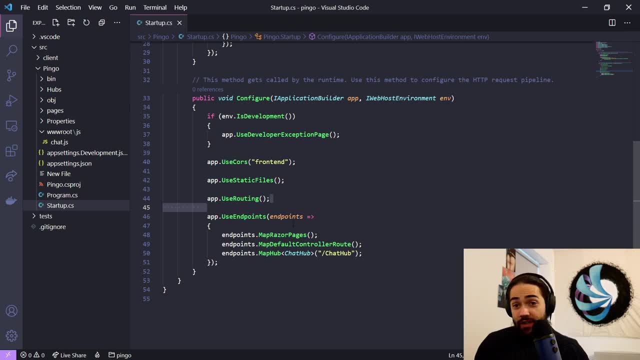 authentication. you can check the state or the context of the headers, look for the tokens in there and see if the user is actually allowed to visit this resource. it can go as far as checking the database, so you can then configure the database to change some values in there and then